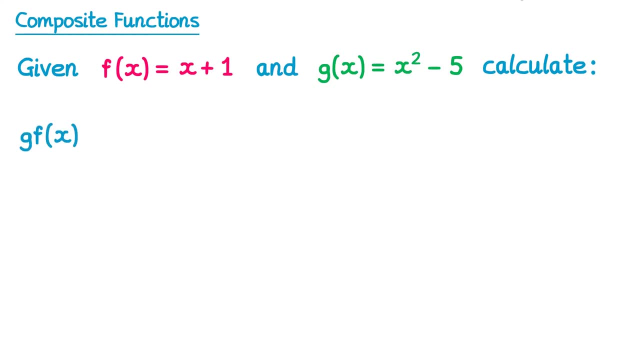 This means we take an input x, we apply the f function to it, which gets f of x, and then we take the output from that and put it into the g function. The best way to write this down is look at your g function first. So g of x is x squared. 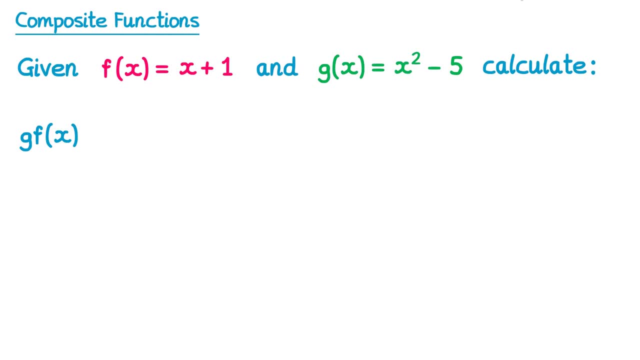 minus 5.. We're going to write that out again, but instead of x's we write brackets, So it would be bracket squared minus 5.. Then inside all of the brackets you write the whole f function. We then just try and simplify this a bit. So x plus 1, all squared is just x plus 1 times. 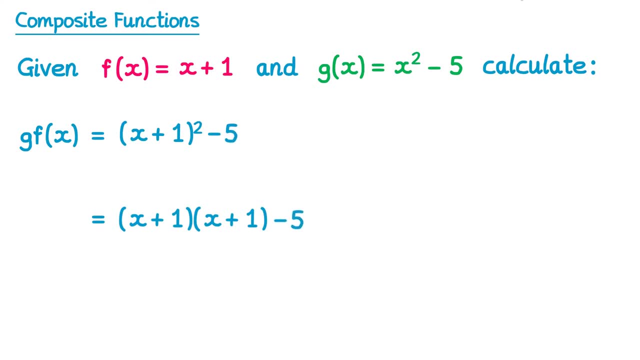 another x plus 1, and don't forget the takeaway 5 at the end. We can expand this using FOIL. so x times x, x squared x times 1, is plus x, 1 times x is plus x and 1 times 1 is plus. 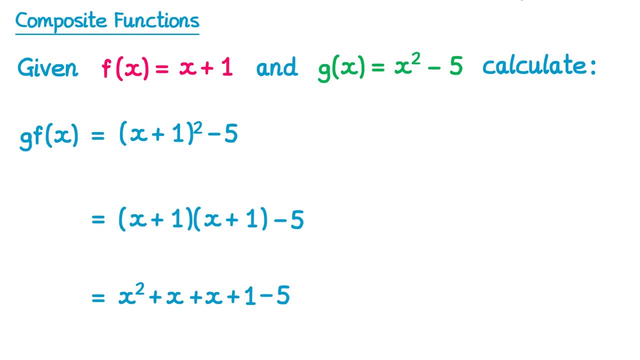 1, and again, don't forget that- negative 5.. We can simplify this, because x plus x is 2x, and plus 1 takes 5, gives you negative 4.. So that's our answer. What if instead it was f, g of x? so the other way around? This means you take an input x. 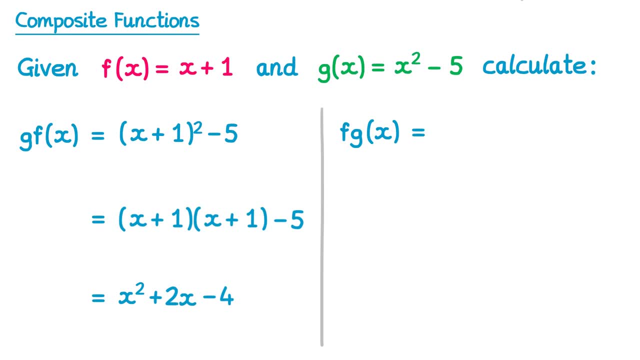 you apply the g function to get g of x and then whatever you get as the output for that you put into the f function. So this time we write out the f function, but instead of x write brackets. So f of x is x plus 1.. 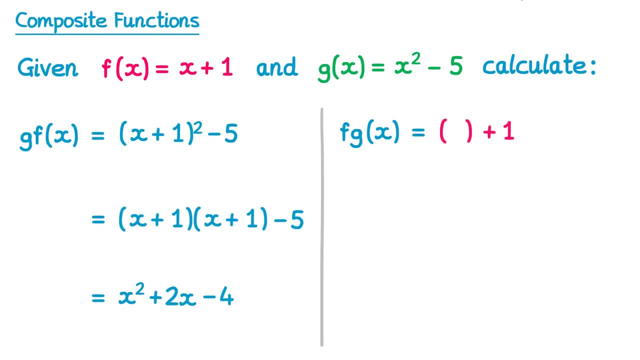 So we'll write bracket plus 1.. Then inside those brackets we put the whole g function. So the g function is x squared plus 5, so that goes inside the bracket. Now we can simplify this one as well. So we have x squared minus 5, and we don't actually 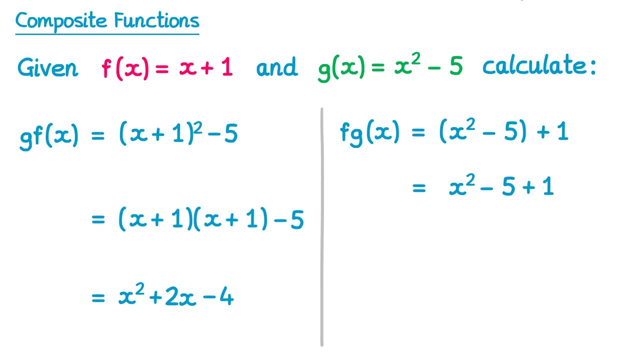 need the brackets here, and then plus 1.. The negative, 5 plus 1, would simplify. so we end up with x squared. take away 4.. Let's try another set of examples now. So we're going to start again with g, f of x.